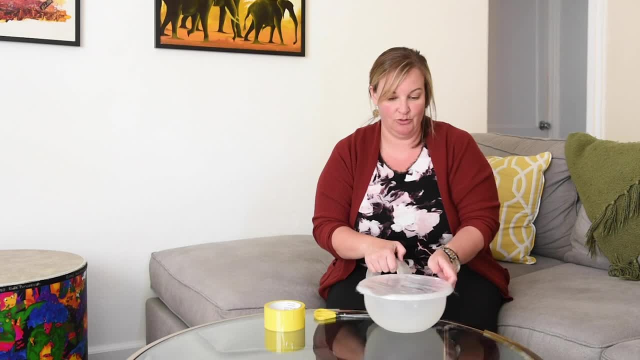 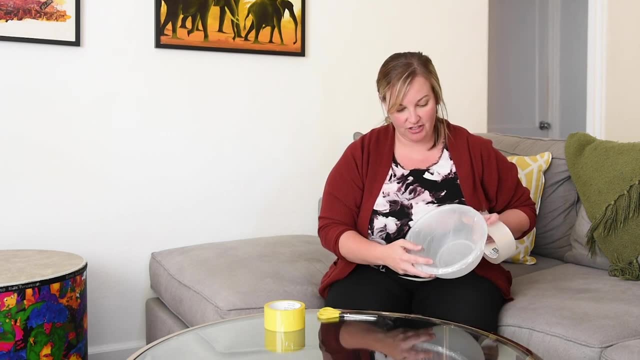 not easy to work with. Making sure you don't lose the end is not easy, but you can do that, So I'm. the end is not easy to work with, so here's our first layer. we've got it going all one direction, as you can see, and so the next thing we need to do in order to add that tension is to go the. 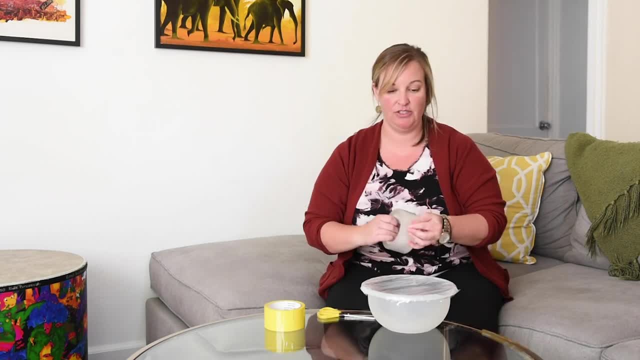 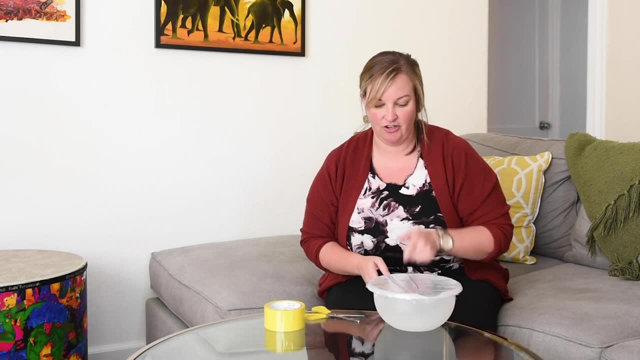 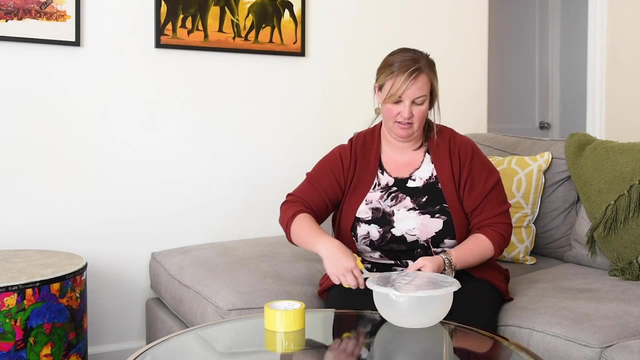 opposite way. so i'm going to take my tape. if it goes this way- now i'm going to go this way- as we add it together, you'll start to notice that your drum head is going to get tighter. so the tighter your drum head, the higher the pitch and you can control to some extent. 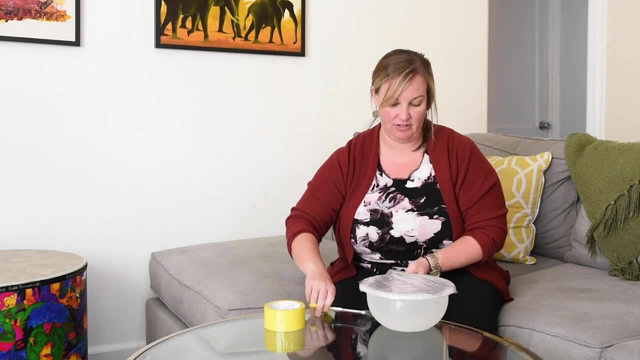 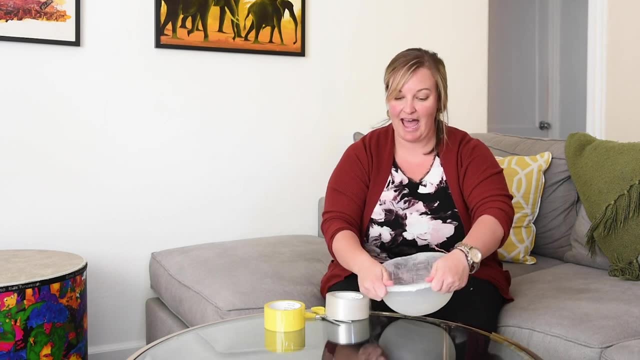 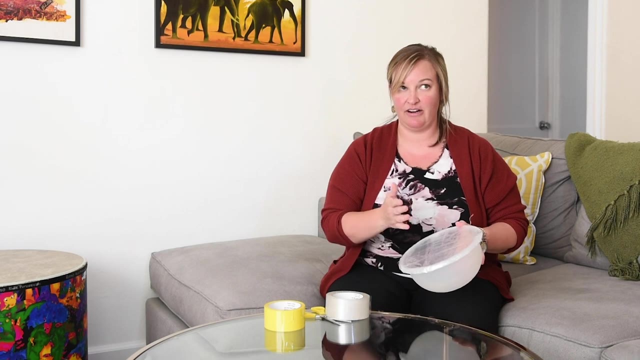 the the pitch level that you get with these drums, meaning the looser the drum head, the lower the pitch. the tighter the drum head, the tighter the pitch, so great. so now i have a pretty tight drum head, uh, going sort of all one way and then all the other way. let's hear how it sounds. 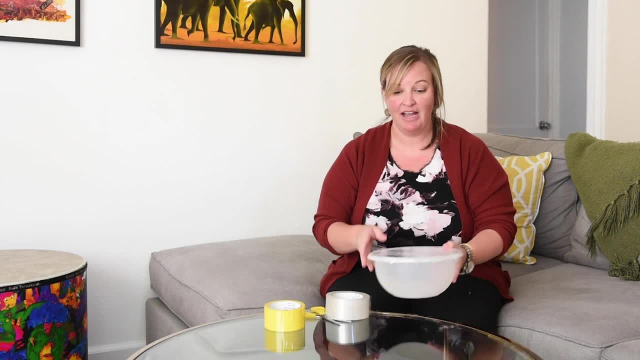 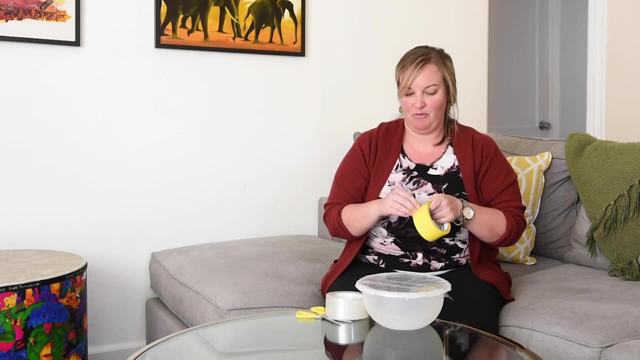 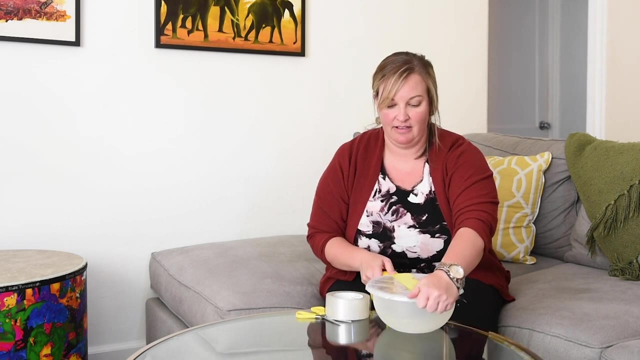 this is not bad. i want to add one more layer of tape. this one i'm going to do sort of a colored piece of tape just to add some flair. why not look like on this wild side? and this one i'm going to take sort of across. and so, since we're getting it across, here's a question: are we adding tension or? 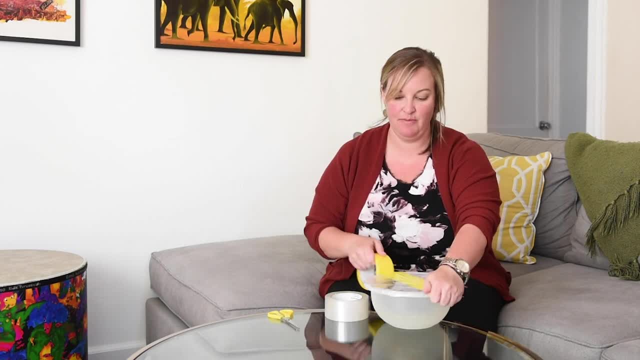 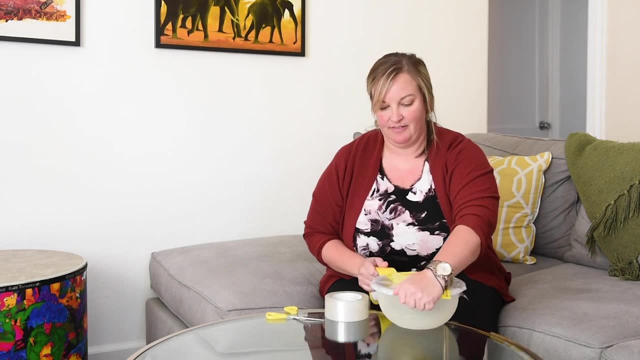 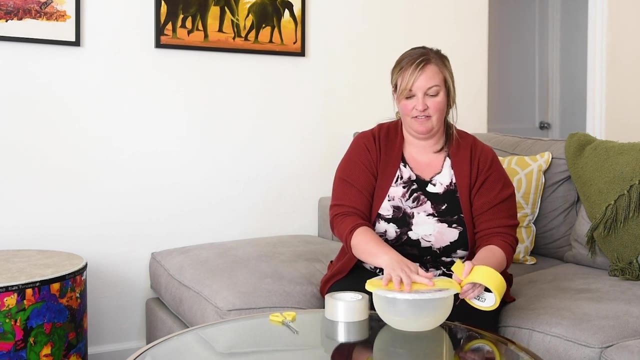 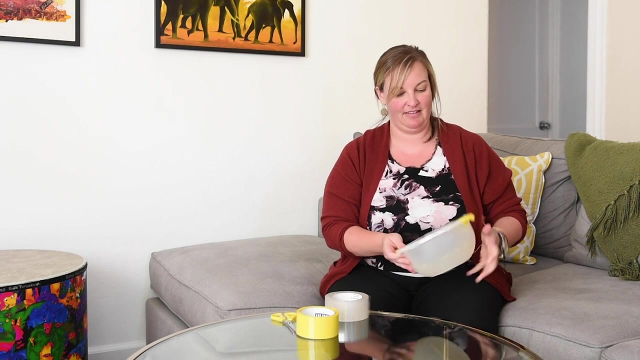 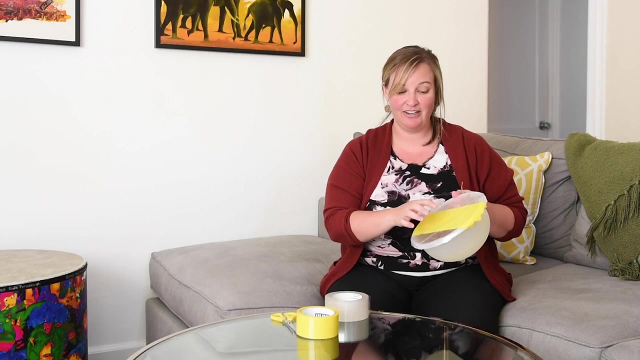 taking it away. tension because we're adding tape. i'm creating in the middle of my drum head here, a place with higher. there we go perfect. look at that beautiful drum. so this is my drum. let's hear what it sounds like in the middle. so if you're listening you can hear. it's just a little bit higher on the side than it is on. 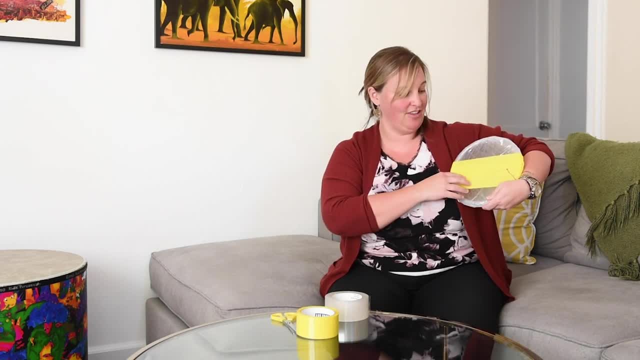 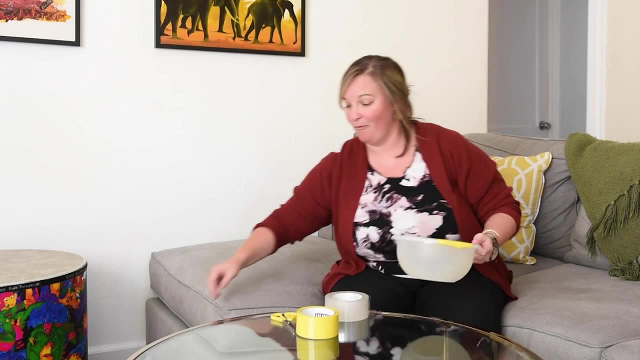 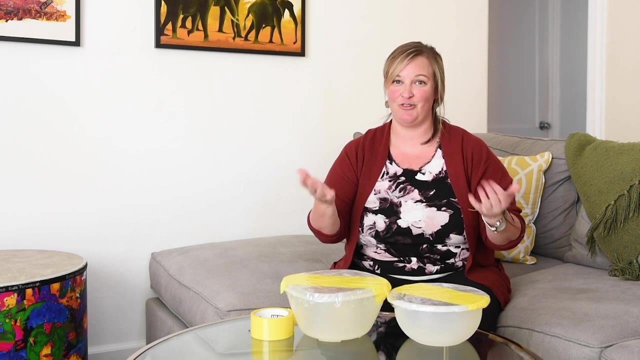 the outside, got a couple different playing techniques. you could throw this right underneath arm, or why not build two and make a drum set and go to town with some pencils or some wooden spoons. so enjoy your drums. thanks for joining us.